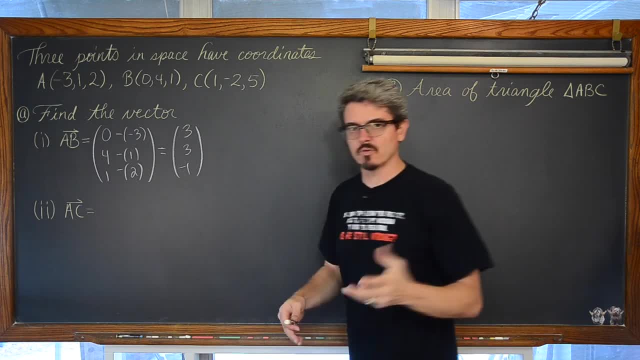 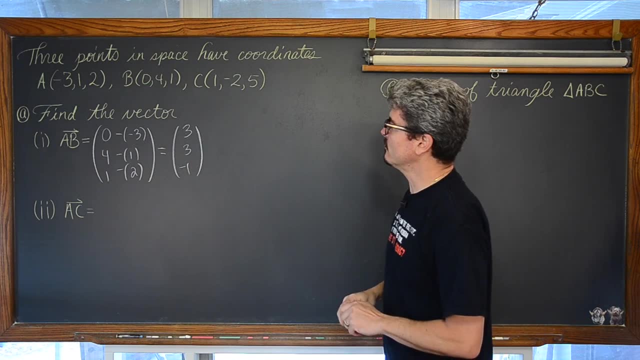 that You might see some arrow brackets and these components moving horizontally. You could also write this as three i plus three j minus one k, If you are doing sort of like that full written form using the component vectors i, j and k in your notation Vector. 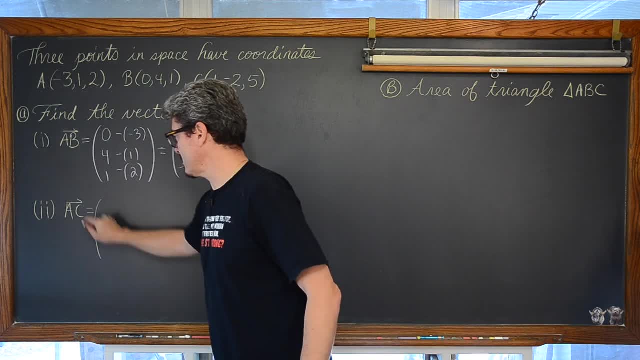 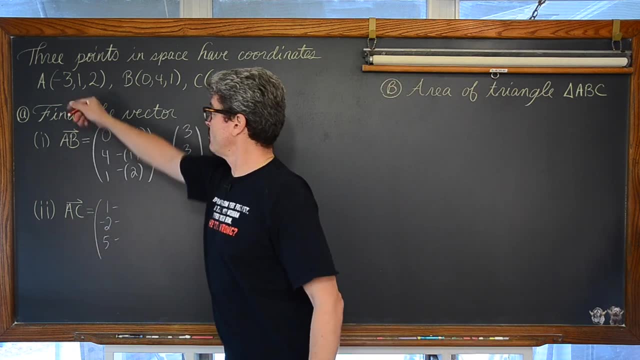 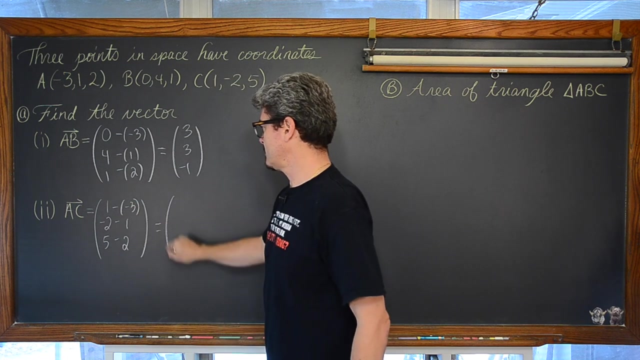 AC, Again, initial point of A, terminal point of C. We will start with the terminal point One: negative, two and five, Minusing with the coordinates of our initial point: Negative three, one and five And two. So we are looking at vaccine. the vector AC has the components of four: negative: 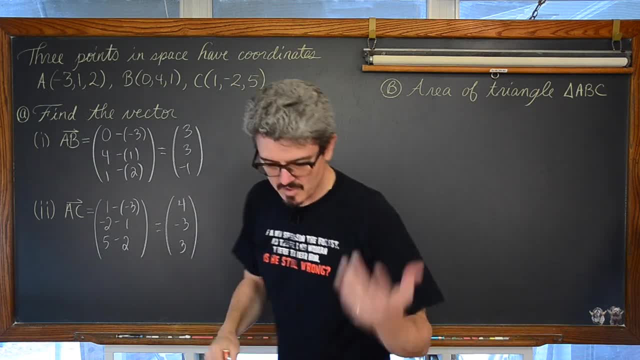 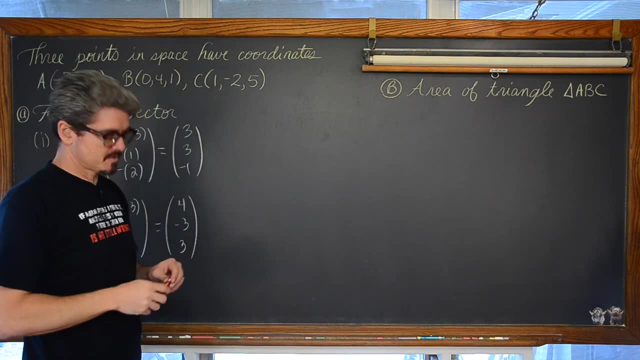 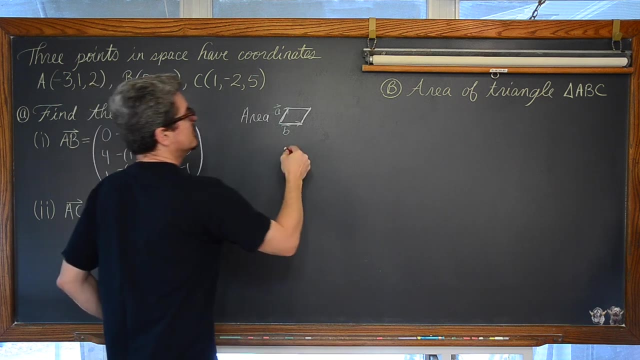 three and three, And just before I go on, make sure I don't make some silly copy error. Now, the area of the triangle defined by these three vertices, working with vectors, So the area of the parallelogram that is going to be equal the magnitude of the cross product. between is equal to vector A. This Washington will be θ, this length will be as n, which is not equals to least n minus one squared x power n squared both times, and as far as the of x comes from the defensive! Fot � is all to the right angle. I will not 3, 2, or 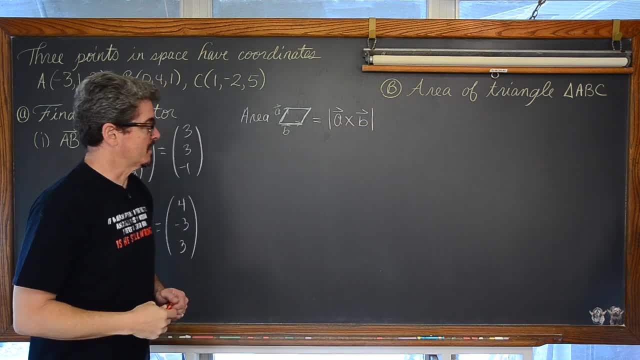 h minus three. Now the area of the triangle defined by these three vertices, working with vectorsWell A and B. Just giving you that as a formula. Well, a triangle is simply half of a parallelogram. So the formula that we are going to use for this triangle is that the area is equal to. 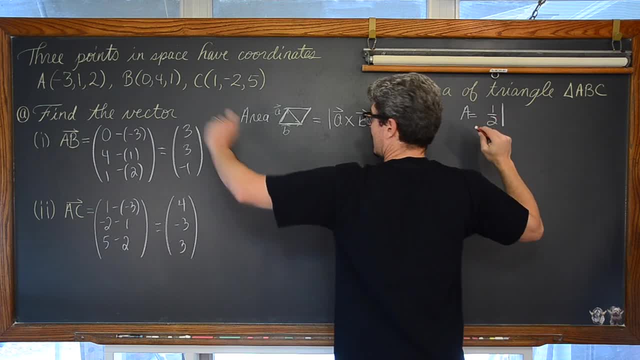 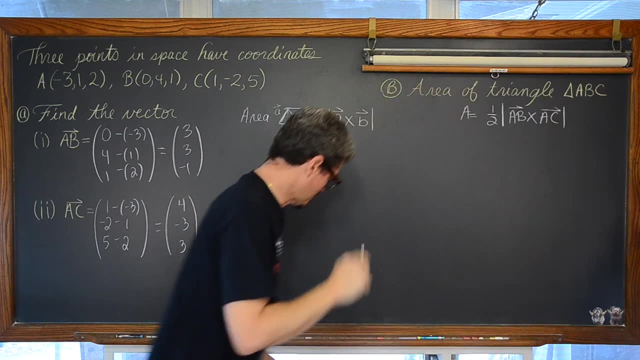 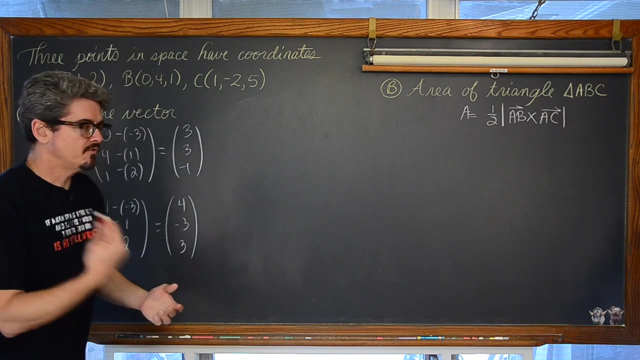 one half the magnitude of the cross product of vector AB and AC. So we are going to find that cross product, that vector- Remember cross product- gives you a vector that is perpendicular to the two vectors that you used to find that cross product with. So cross product of AB. 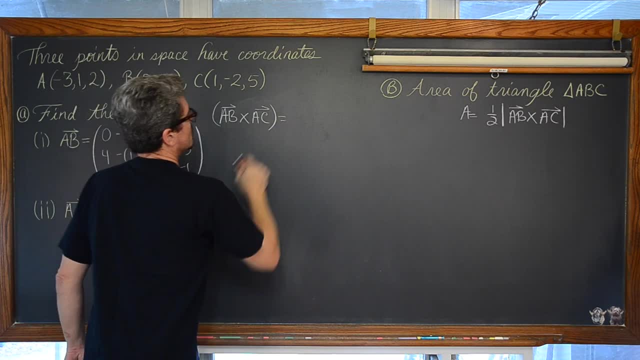 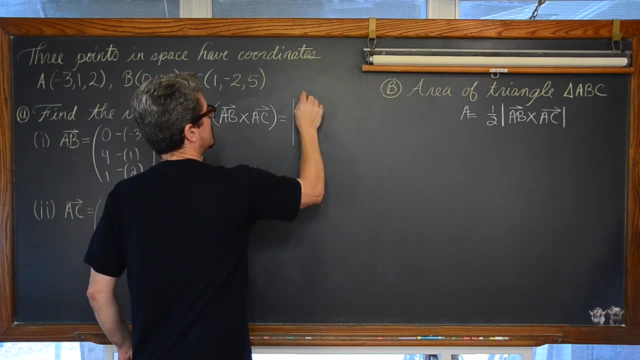 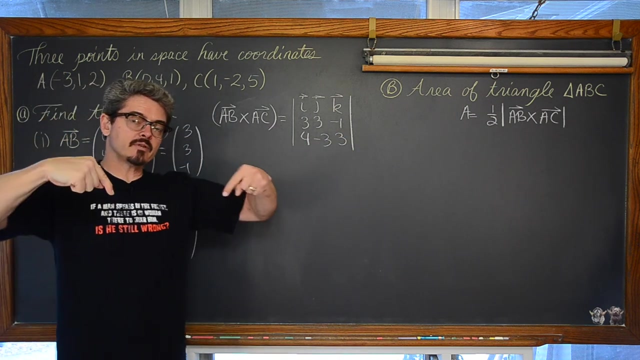 and AC. We are going to basically take the derivative, the determinant, excuse me. we are going to set up a component row i, j and k And then make a row below with the components from vector a and c I talk about in the video. I have a link. 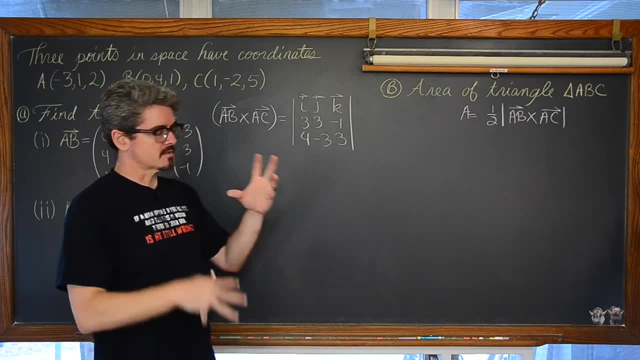 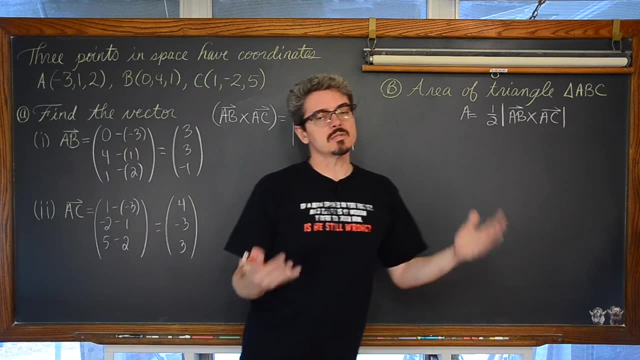 in the description that the cross product is not commutative. If you reverse this order, you get an opposite answer. But we are going to be ultimately working with the magnitude, which is length. so that is not an issue for us here. We are going to be looking for the 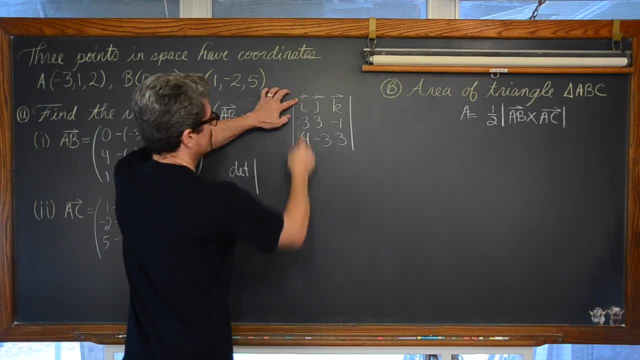 determinant of the 2 by 2 matrix, taking out the row and column that has this component vector i in it. We are looking at 3, negative 3, negative 1, and 3. That is going to create a coefficient for the component vector moving in the direction of the x axis Minus so 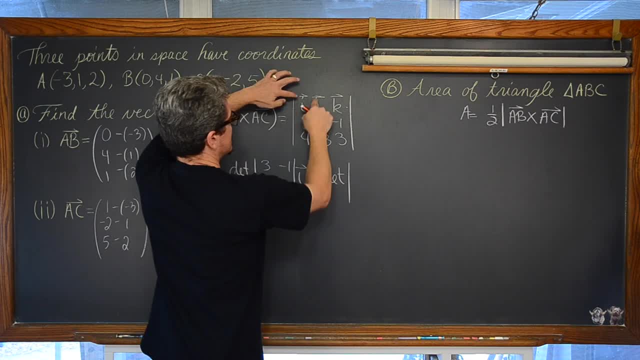 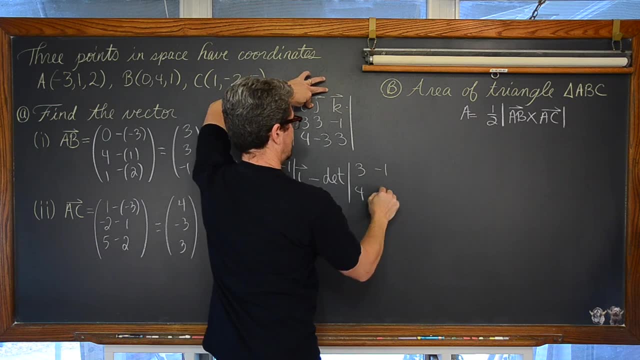 we have a plus, minus and then the determinant. Take out the column and row that has the component vector in the direction of the y axis, So 3,, 4,, negative 1, and 3.. Add that with the determinant. I am just writing this in here to really make sure that you realize that. 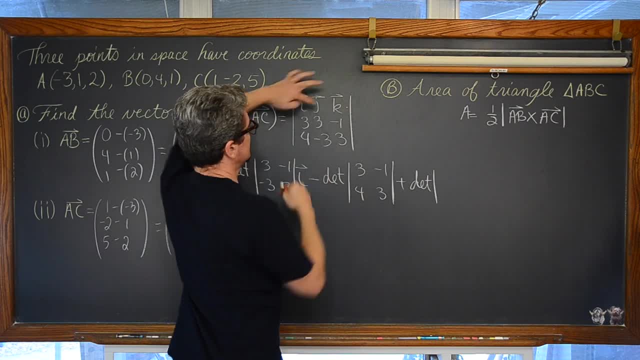 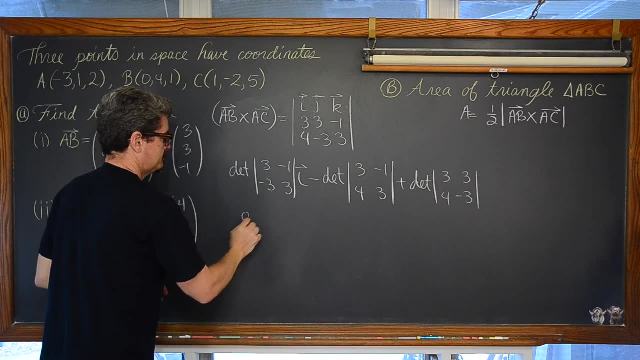 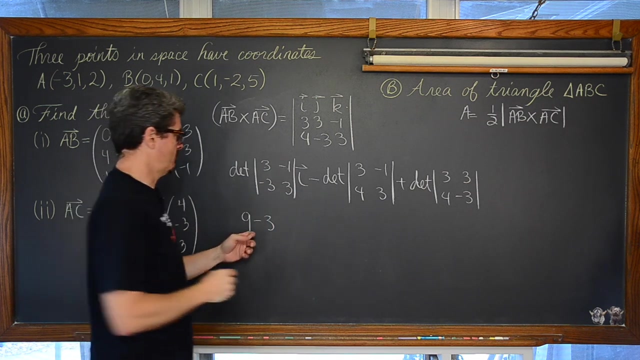 that is what I am looking for. Take out the column and row with the component vector in the direction of the z axis. Now we are looking at 9 minus 3.. So 3 times 3 is 9.. Then minus the product of negative 3 and negative 1. That is going to be a coefficient of negative. 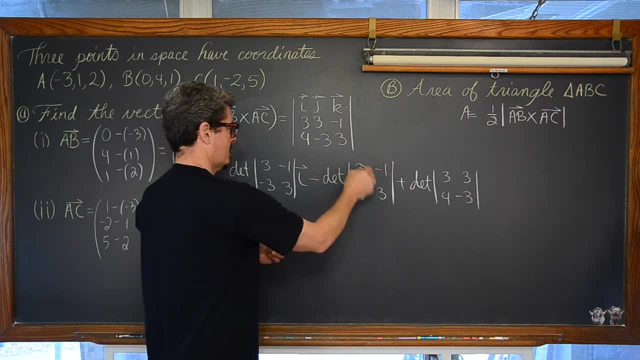 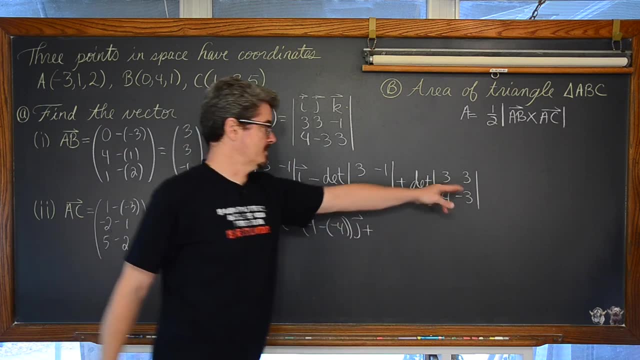 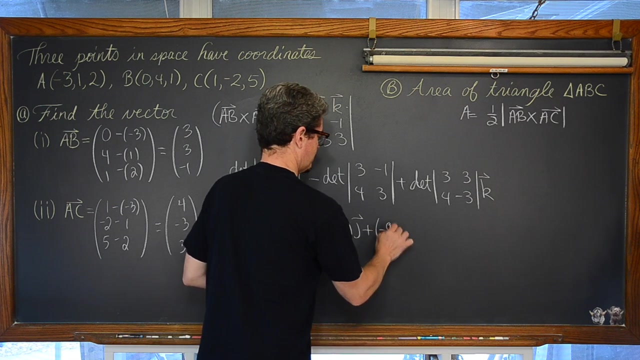 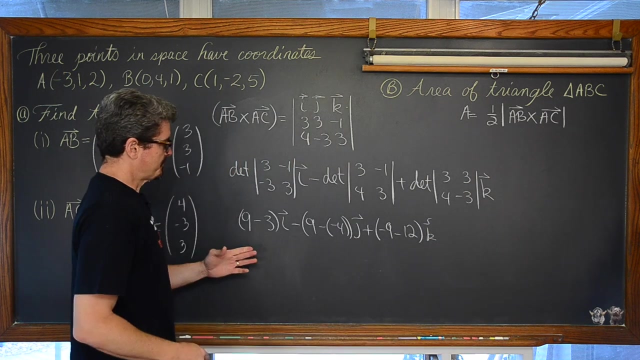 3. That is the determinant of vector i Minus. we have got 9, minus negative. 4. The determinant of this 2 by 2 matrix, which should have a little vector k over. here We are looking at negative 9 minus 12.. That is vector k, So our cross product is equal to 6 minus 12.. 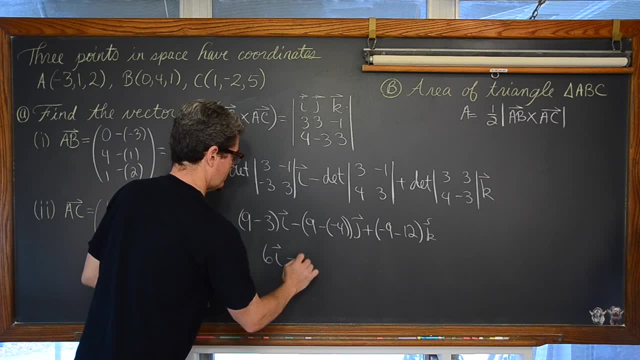 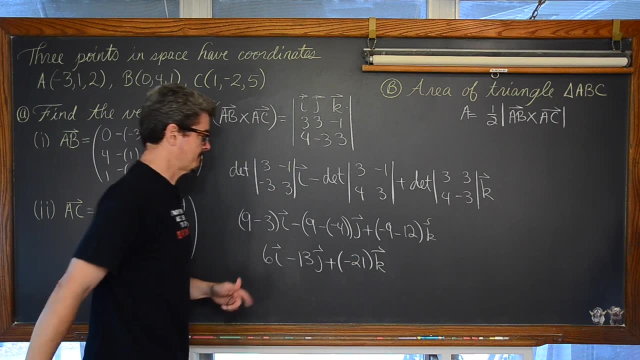 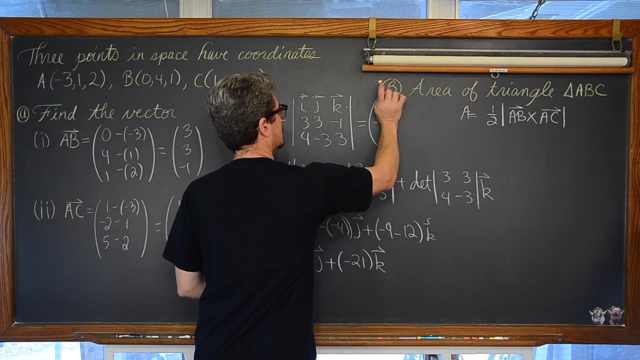 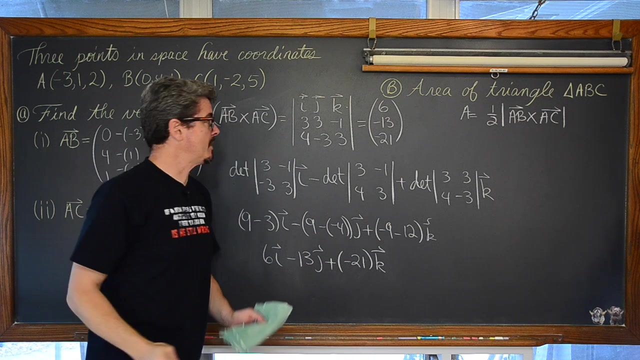 Then we have got minus 12 and i minus 13j, plus negative 21. vector k, Or the cross product, is equal to 6, negative 13, and negative 21.. I got to this point after I made this problem up and realized that my numbers are a little bit gross. This was really intended to be.